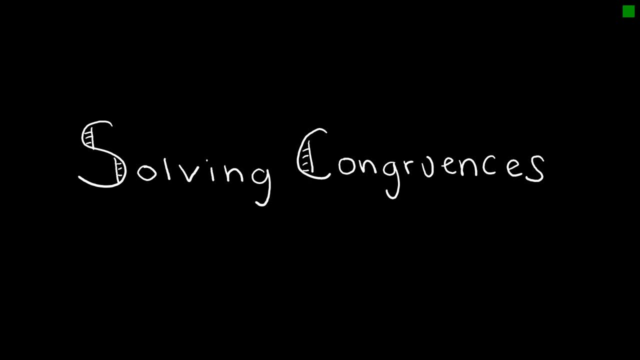 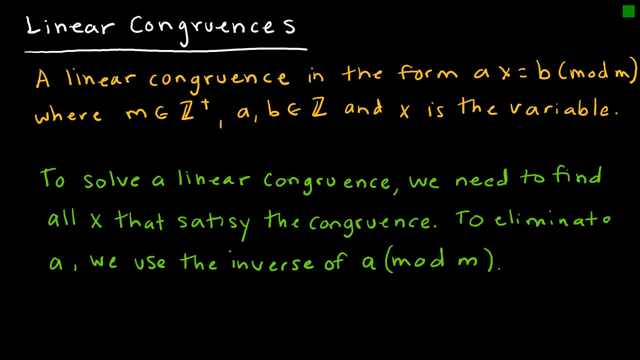 In this lesson we will look at solving congruences. So a linear congruence is in the form AX equal B mod M. So we're looking at modular division, and what we haven't seen up to this point is we haven't seen a value A in front of our 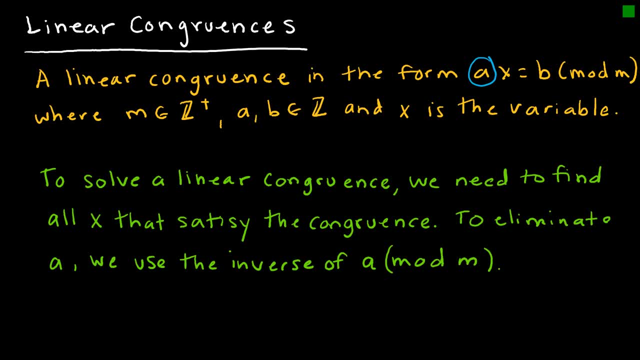 expression. So we're saying mod M, A and B are integers and X is the variable. and to solve this, essentially what I'm looking for is all of the X's that will satisfy the congruence, And so what I want to do, just like in a normal 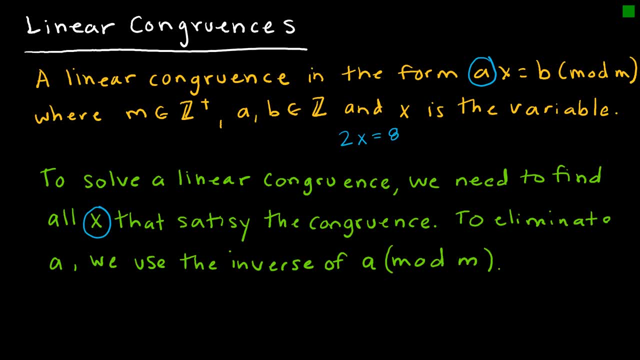 equation. if I said, you know, 2X equals 8, we would be solving to find that X is 4, and that would be the only X that satisfies the equation. What I'm looking for is essentially to try to eliminate the A, because then I would be left with 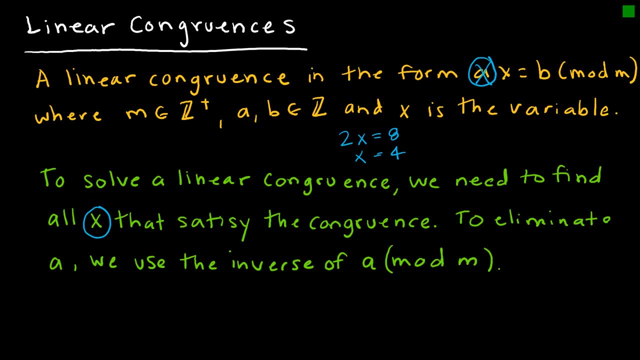 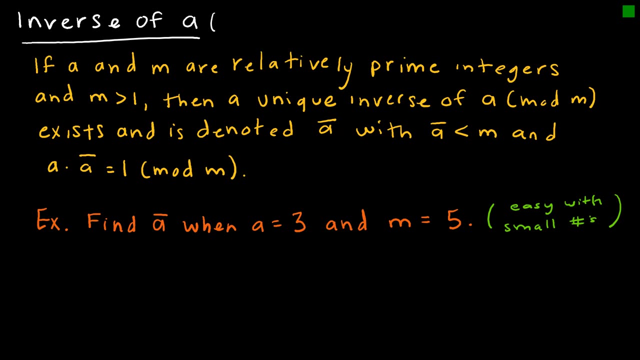 you know, X equal B mod M, And we know how to handle that situation. So, in order to eliminate the A, we must learn how to find the inverse of A mod M. So what is the inverse of A, or I should have said what is the inverse of A mod M? Well, if A and M are relatively prime, 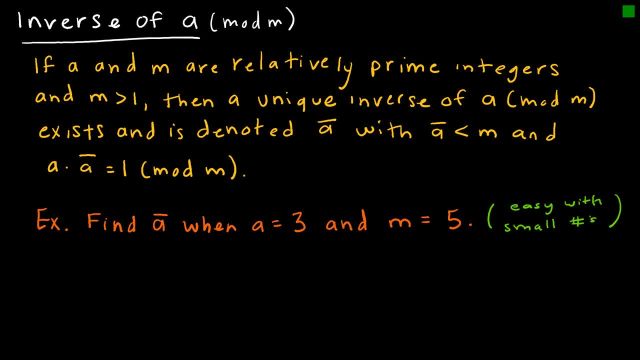 integers. so what does that mean? Relatively prime means that A and M don't have any factors in common And M is greater than 1, then a unique inverse of A mod M exists and is denoted with a bar. So that would be the inverse of A, and the inverse of A is going to be. 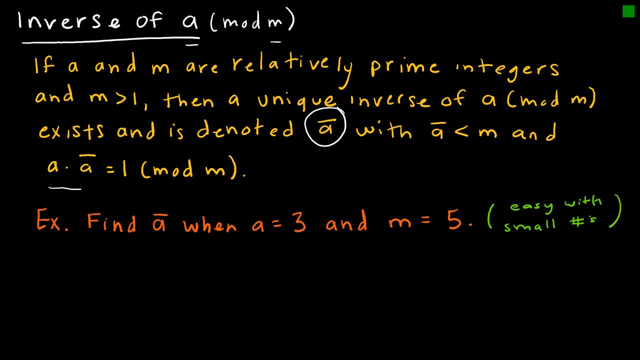 less than M. and if I took A times the inverse of A, I should get 1 mod M. So what does this mean? Well, if I'm dealing with some small numbers like, say, A is 3 and M is 5, then I can just say: well, 3 times what is going to give me a? 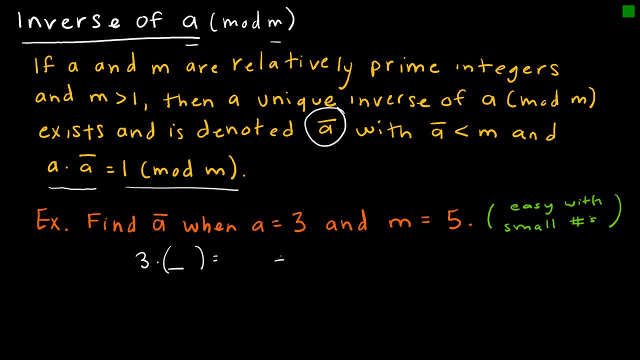 remainder of 1.. That's exactly what I'm looking for, mod 5.. So essentially I'm saying: if I divide by 5, so 5 times what would give me that remainder of 1? and so here I can see: well, if I took 5 times, if I took 5 times, 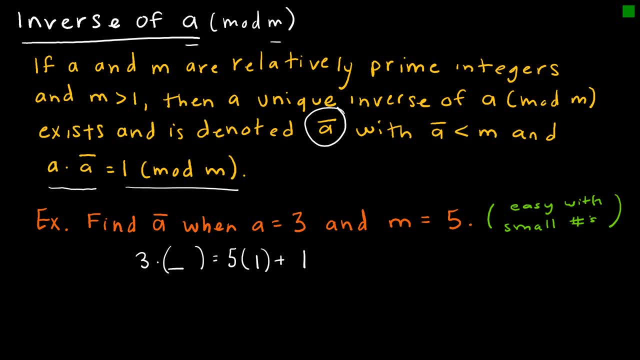 1, 5 times 1 would be 5 plus 1 is 6, and 3 times 2 is 6. so I know that the inverse of a in this case is 2. I could have also done that with a different number, so I. 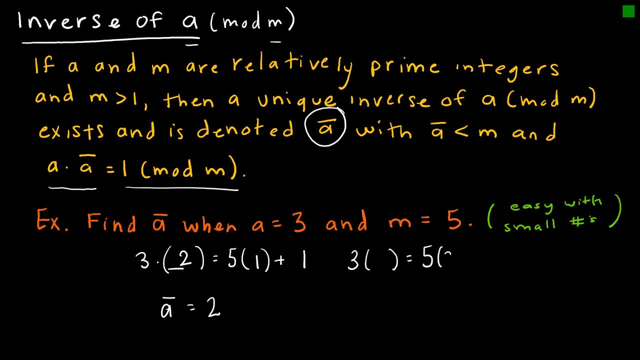 could say 3 times what? and what if I said 5 times 2 plus 1? well, 5 times 2 plus 1 is 11, and 3 doesn't go into 11. so that's not going to work, and so I could. 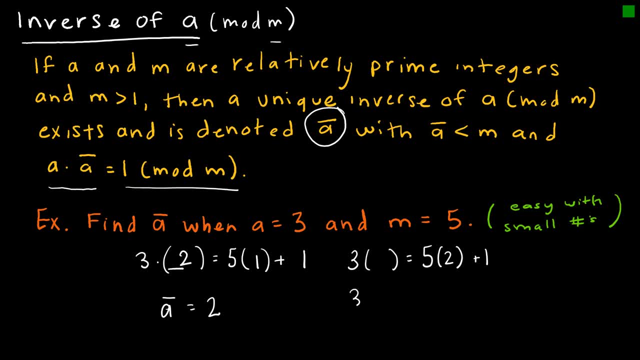 find other values that do in fact work. let's say 3 times. I'm going to cross this one off 3 times. what equals 5 times 3 plus 1? well, 5 times 3 is 15 plus 1 is 16, so that one's not going to work. 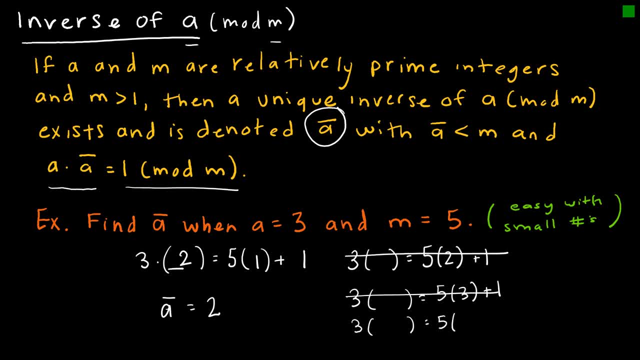 I could look at 5 times 4, and 5 times 4 plus 1 is 20 plus 1 or 21, and that one does work. so 3 times 7. so I can also say that an inverse of a is 7. but just as we 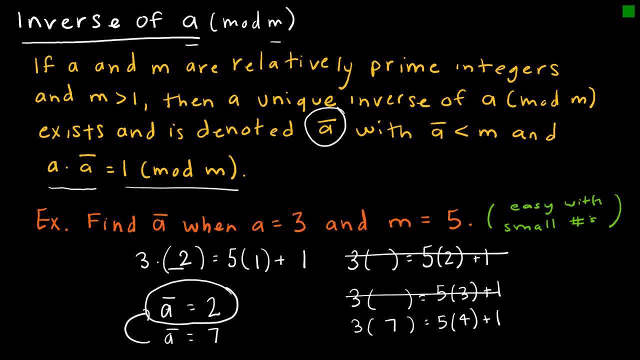 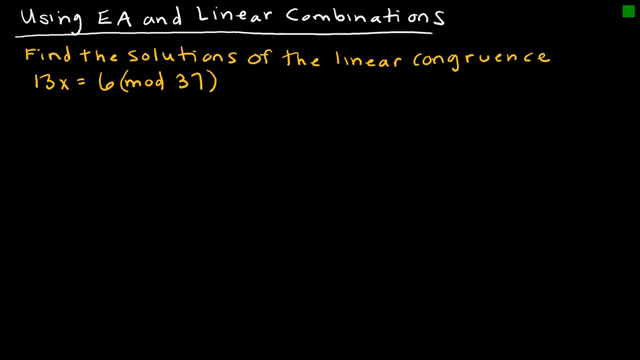 did before. what I'm looking for is that smallest one, because 7 and 2 are the same mod 5 or equivalent mod 5. so let's take a look at an example using the Euclidean algorithm and linear combinations, and this should look super familiar to us because we've done this. 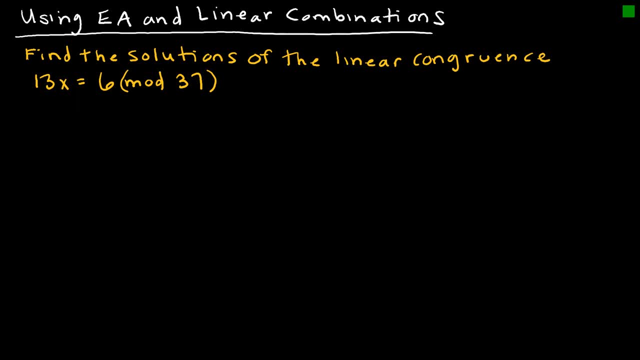 several times, but the first thing that I need to do is I need to show that the GCD, the greatest common divisor of 13, which is my a and 37, has to be 1. now, why does that have to be true? Now, why does that have to be true? 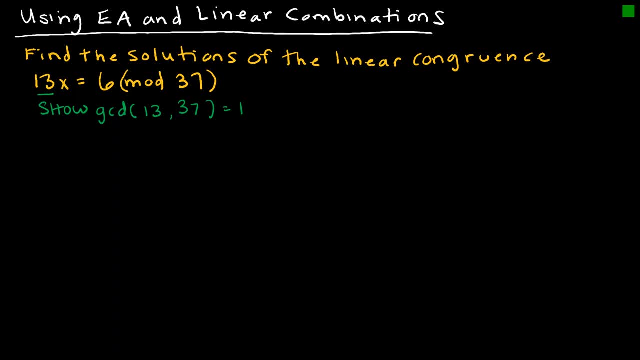 because in our definition we had said that the two values must be relatively prime, which means their greatest common divisor needs to be 1. so how can I show that? I can show that using Euclidean's algorithm. so 37 equals 13 times 2, which. 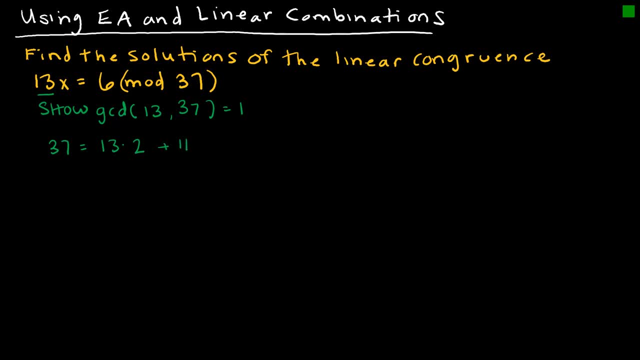 is 26 plus 11, so 37 equals 13 times 2, which is 26 plus 11, and then 13 equals 11 times 1 plus 2, and then 11 equals 2 times 5 plus 1 and 2. 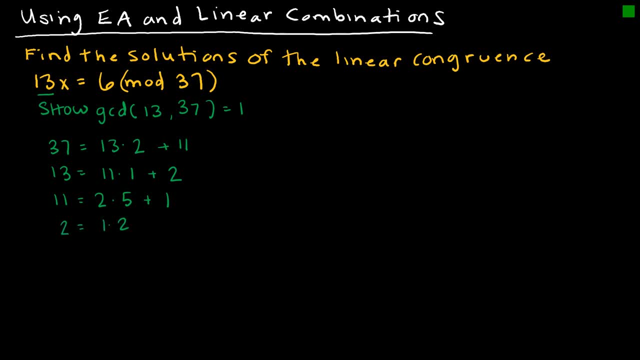 equals 1 times 2 plus 0, and so therefore, I have determined that it is an fact. 1. so that is the first step. show that they are relatively prime. now we're going to do just as we did before, so we're going to start backwards and work. 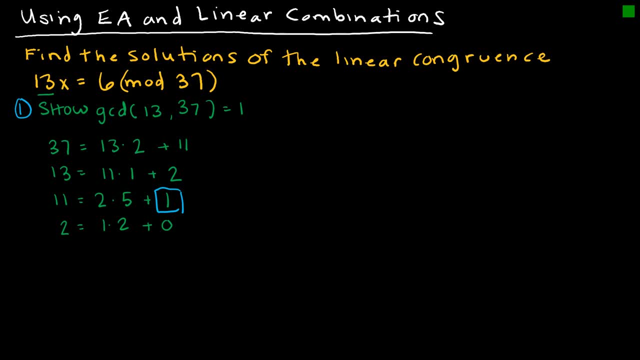 our way through. so again, I can write this as: 1 equals 11 minus sorry, 1 times 11 minus 2 times 3 minus 2 times 3, or I guess I should write 5 times 2, since I'll be replacing the two, and then 2. 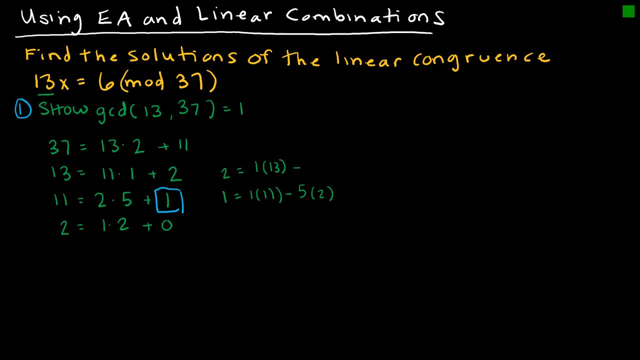 equals 1 times 13 minus 1 times 11. and then 11 equals 1 times 37 minus 2 times 37 minus 2 times 3 times 13.. And again, I'm going to do this as I did before, just doing a lot of substitution. 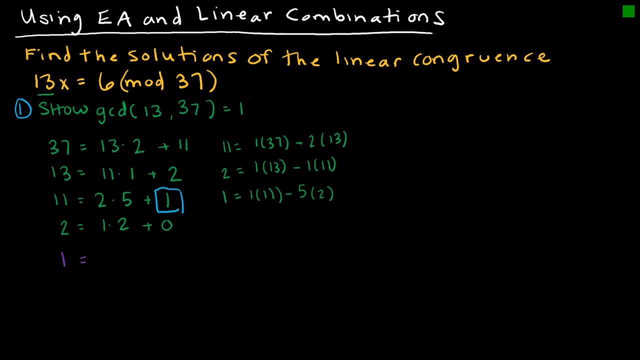 And so I'm going to start out with one equals, So again, one equals. and I'm going to write one times 11 minus five, And instead of two I'm writing what two is equivalent to using this. And again, I'm just interested in how many groups of each thing I have. 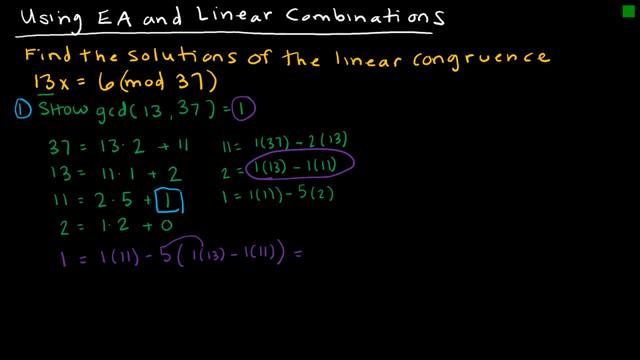 So I'm going to take negative five times one that gives me negative five groups of 13. And negative five times negative one gives me positive five plus one which gives me positive 12.. 6 groups of 11. And then I'm going to continue the process. So I still have 1 equals and I have 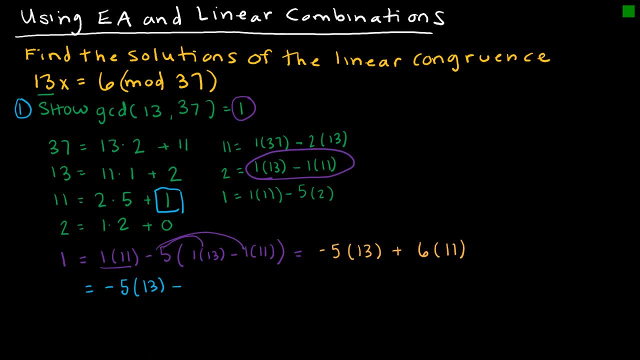 negative: 5 times 13 plus 6 times what is equivalent to 11,, which is 1 times 37 minus 2 times 13.. And then I'm going to simplify. So again: 6 times 1 is 6.. So I have 6 groups of 37.. 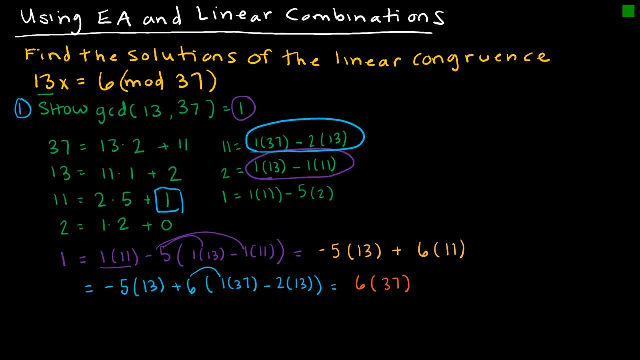 And then I take 6 times negative 2,, which is negative 12.. 6 times negative 2,, which is negative 12, plus negative 5 is negative 17. So I get plus negative 12. So I have 6 groups of 37. And then I take 6 times negative 2,, which is negative 12.. 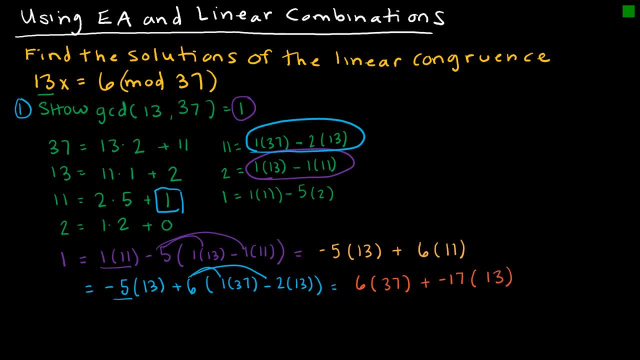 And then I take 6 times negative 2, which is negative 17 groups of 13.. So how has this really helped us? Because we've done all of this before, right. So what we have right now I'm just going to recopy up here. I have: 1 equals again 1, because that was the 1 here. 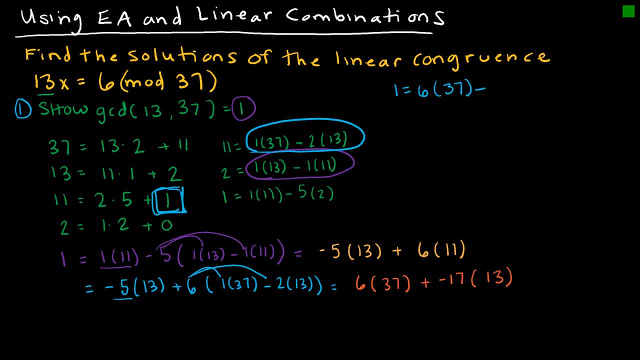 1 equals 6 times 37, plus negative 17 times 13.. So what I'm looking at here is I'm looking at a mod 37. And if I'm looking at mod 37, then I know that 37 and any multiple. 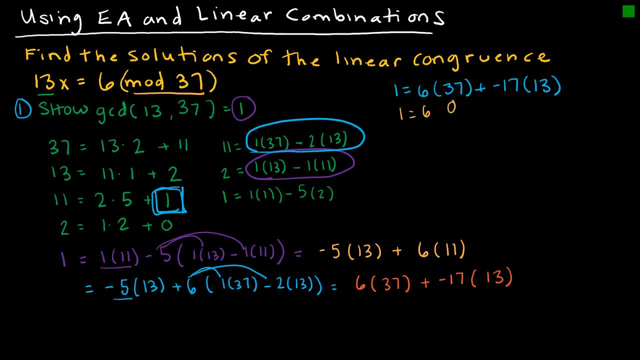 of 37 is actually equal to 0. So I have: 1 equals 6 times 0, plus negative 17 times 13. And that tells me that if I do some reduction, that 1 is equal to negative 17 times 0.. 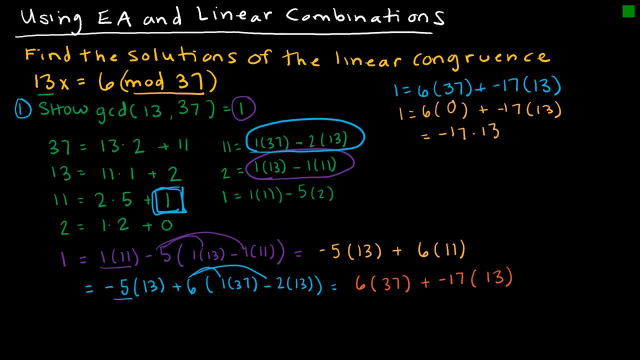 I'm sorry, I should have specified: 1 in mod 37 is equal to negative 17 times 13.. So what does that tell me? That tells me that negative 17 is an inverse. So we said that we had to solve this. 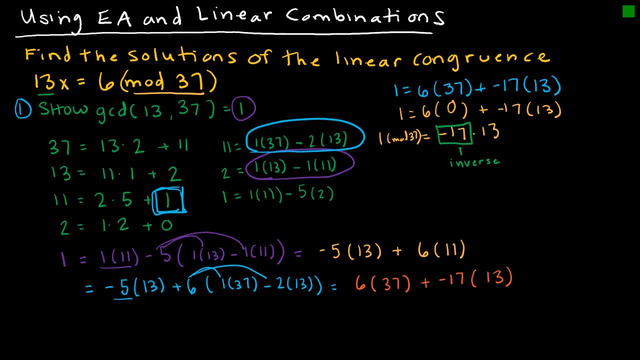